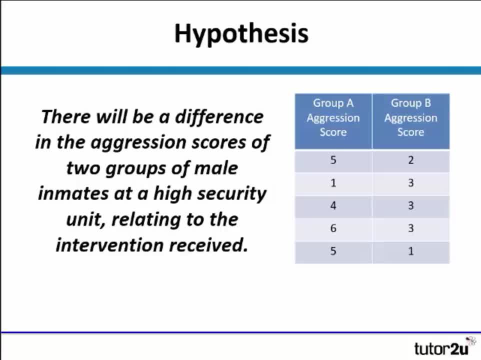 relating to the intervention received. So we have two groups, as you can see. We have group A and their aggression scores and we have group B and their aggression scores. So to test the difference, we're looking at the difference between them. We're also going to look at two completely separate groups. 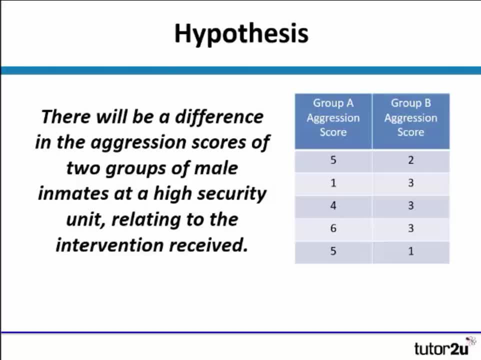 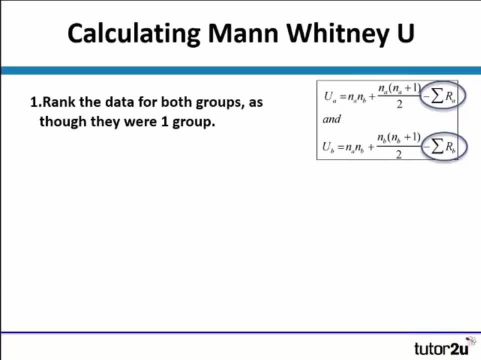 so group A and group B are independent measures and the data is at least ordinal. So the first thing that we need to do for calculating Mann-Whitney is to rank the data for both groups as though they were one group, And this has been done for you already. 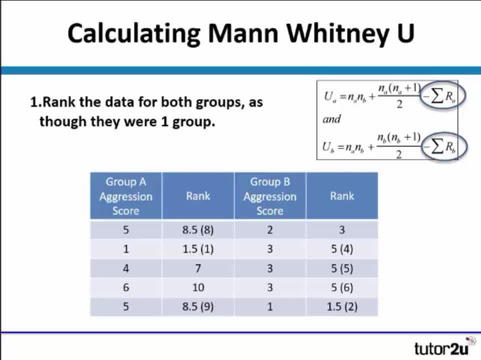 Now I want to look carefully at the table, because the ranking process is quite complex. So, as you can see, we have two scores of one. Okay, so we have two scores of one. They would respectively receive the rank one and two. However, because they are the same score, they have to receive the same rank. 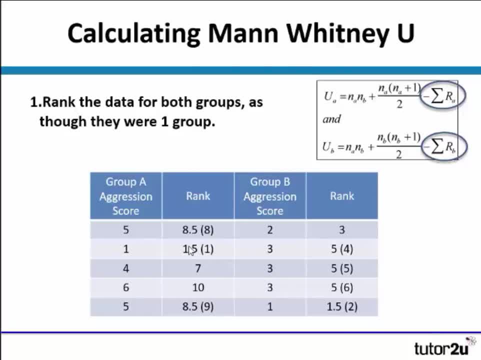 So the difference between one and two is 1.5.. So instead of getting ranks one and two, they get 1.5, which is the midpoint between the two. So that's rank one and rank two gone, Which means our next number is 2.. 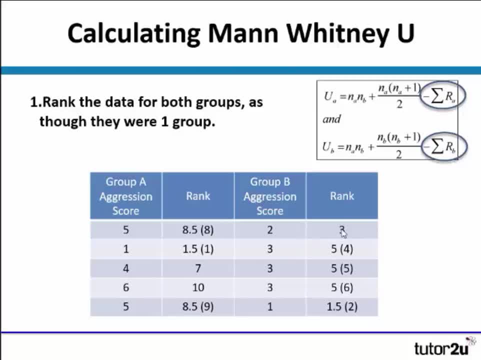 Our next number will take rank three, As there is only one score of two. that's fine. We then have to look at what would get our fourth rank, And we can see that would be three. However, we have three threes. 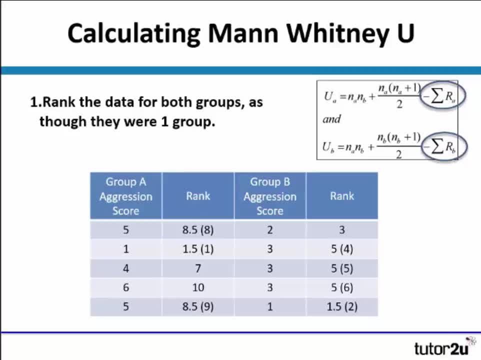 So similarly we have to give them equal ranks. So rank four, five and six are where those three positions would be, But they have to have the same number. The middle number between four and six is five. So all the three are equal. 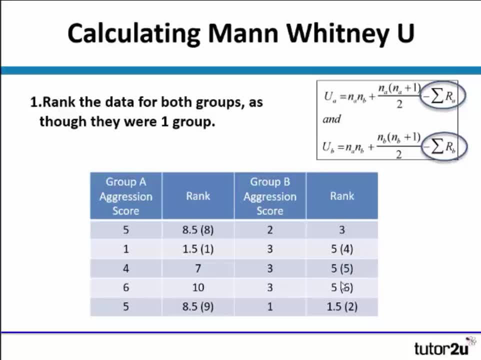 All the threes get a rank of five. We're now up to rank seven. There's only one, four, So that gets rank seven. We then have to look at fives. We've got two of those, So they would take ranks eight and nine. 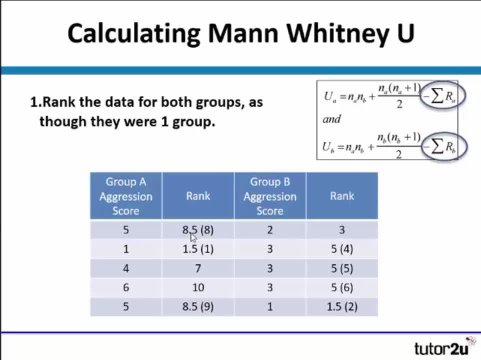 Again, because there are two of them. they have to take the middle position, So it's 8.5.. And then we only have one sixth, So that would take rank ten: One, two, three, four, five, six, seven, eight, nine and ten. 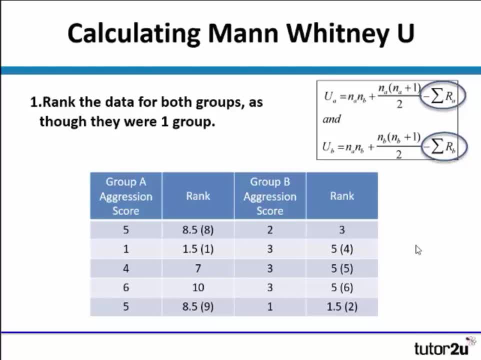 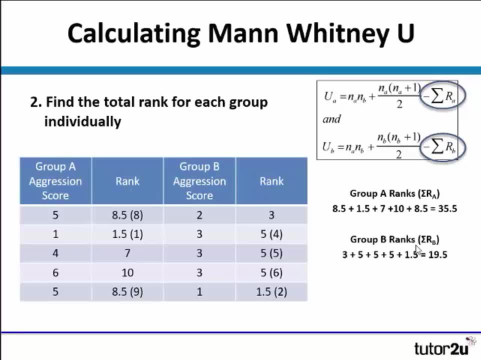 But we've divided up the ranks where there are two scores that are the same. The second part of Man Whitney U is to find the total rank of each group individually. So now we've ranked them as a whole group. We now need to look at the scores that group A got and the scores in the ranking that group B got. 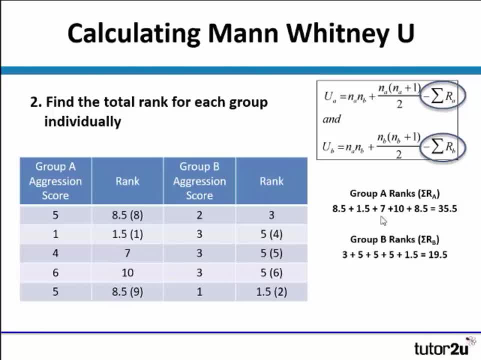 The 8.5 add 1.5,, add 7,, add 10, add 8.5.. By my calculations it's 35.5.. And then 3, add 5,, add 5,, add 5,, add 1.5.. 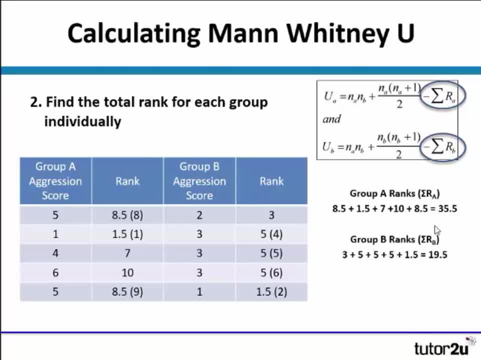 Again, by my calculations it's 19.5.. And this is symbolized by sigma rA and sigma rB, which you can see here in the formula. That simply means the total of the ranks of B and total of the ranks of A. 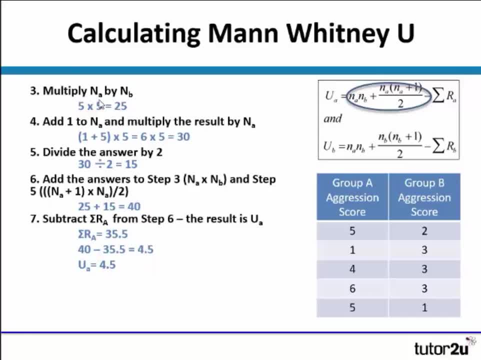 So the next couple of steps are quite straightforward. So we have to multiply, as you can see in the formula, nA by nB. Now we have five participants in each group, So 5 times 5 is 25.. The next part: if we look at the formula, we have to add 1 to nA and times that by itself. 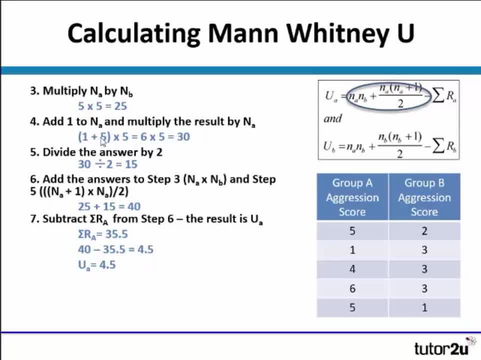 So 1 add 5 times by 5.. So 1 add 5 is 6 times 5 is 30.. And then the last little bit: here we have to divide that answer by 2. And that gives us 15.. 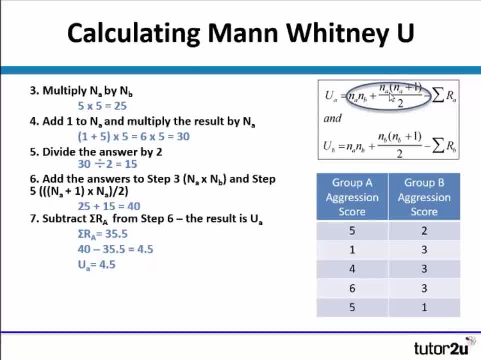 So we've calculated this section here. We've calculated this section here, But you can see there's an addition sign, So we need to add the two together. So 25 add 15 is 40.. We then need to subtract sigma rA, as you can see from this part of the formula. 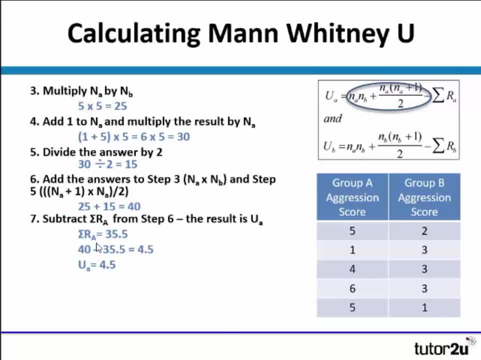 from what we've just calculated, And this would give our answer for uA. So sigma rA is 35.5.. 40. Take away 35.5 is 4.5, which gives us a score of 4.5.. 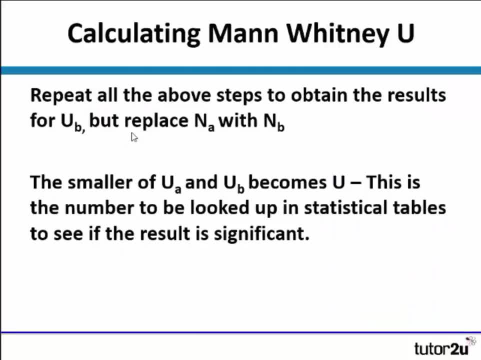 We then have to do exactly the same for uB, our group B, But we need to make sure that where it says nA, we replace that with nB And the smaller of the two calculated scores becomes the u value which we would look up in the statistical values table. 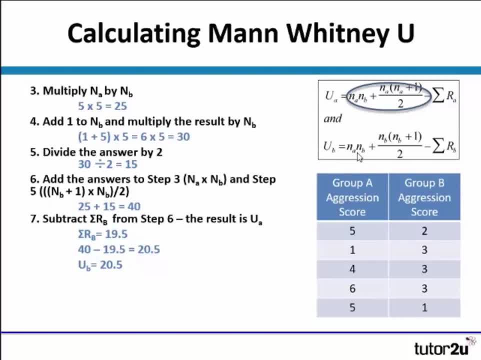 So if we have a little look at this, So we're now working on uB, So nA times nB Is still 25.. Add 1 to nB. Well, we've got the same amount of people in the group. 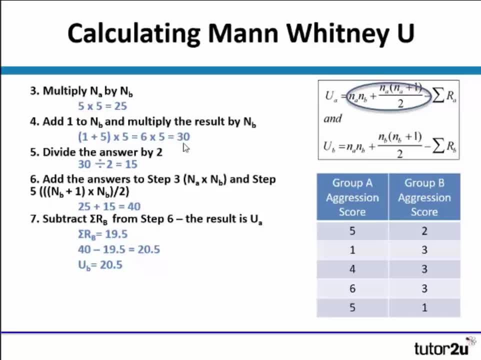 So 1 add 5 is 6.. Times by 5 is 30. We divide that answer by 2, which gives us 15.. 25 add 15 is 40. And then the final bit: we subtract sigma of the sigma rank scores B from the result. 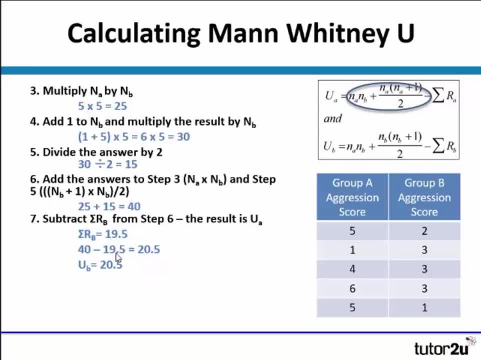 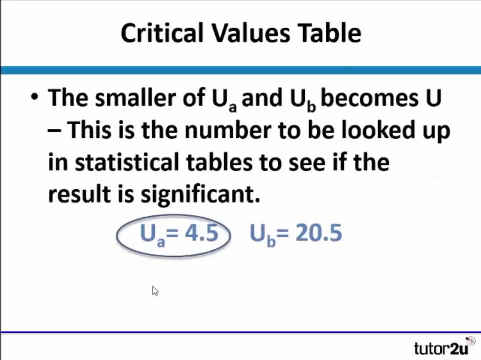 And our sigma rank score was 19.5.. So 40 take away 19.5 is 20.5.. And this becomes uB. So in terms of looking up the data in the critical values table, the smaller of uA and uB becomes u. 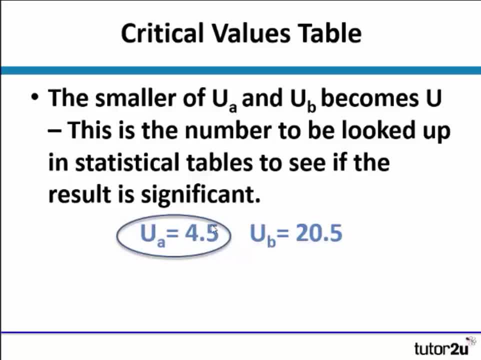 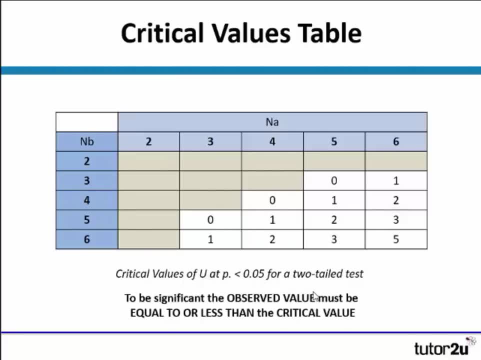 So we only look at one score in the statistical values table And we just take the smaller one of the two that we've calculated, So 4.5.. So here we have a very small snapshot of a critical value table, And it's at 0.05.. 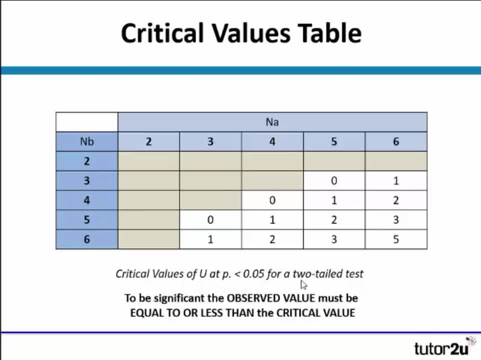 So we're looking at the probability of our results being due to chance at about 5% And because we had a two-tailed hypothesis, we're obviously using a two-tailed test. So to be significant, our observed value must be equal to or less than our critical value. 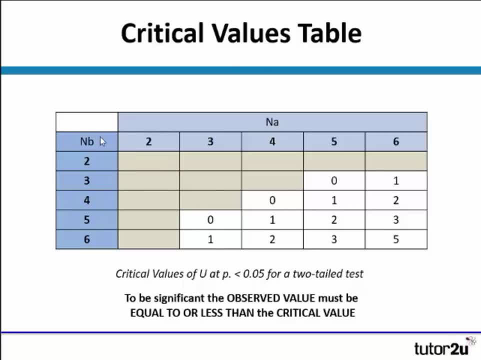 So how do we look this up? Well, we need to look at nA and we need to look at nB. Both of those had five participants, So the score that our observed value needs to be smaller than is 2.. Well, our value was 4.5. 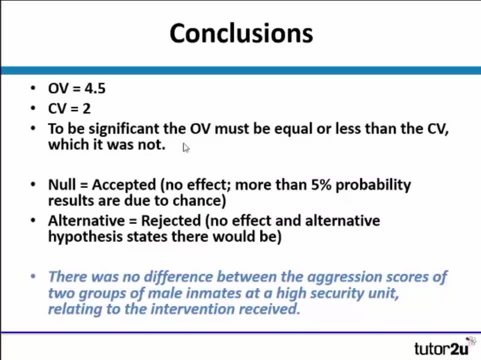 So what does that mean? Well, that means it was not significant. To be significant, our observed value needed to be equal or less than our critical value, which it wasn't. So because this is the case, we accept our null hypothesis because there was no effect. 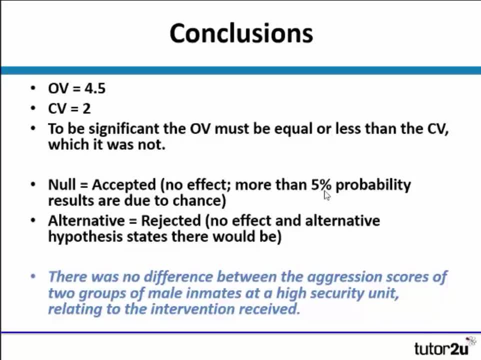 And this simply means- because we tested it at p.05, that there was more than a 5% probability that the result was due to chance. Because we've accepted the null hypothesis, we need to reject our alternative because there was no effect.